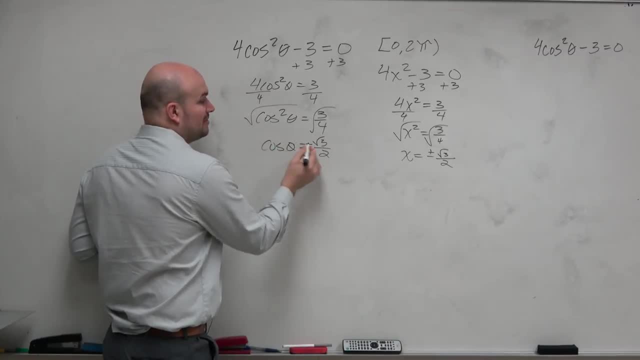 When I take the cosine of that angle, I get square root of 3 over- I'm sorry, plus or minus right. Plus or minus square root of 3 over 2. And then I have my constraint: 0 to 2 pi. 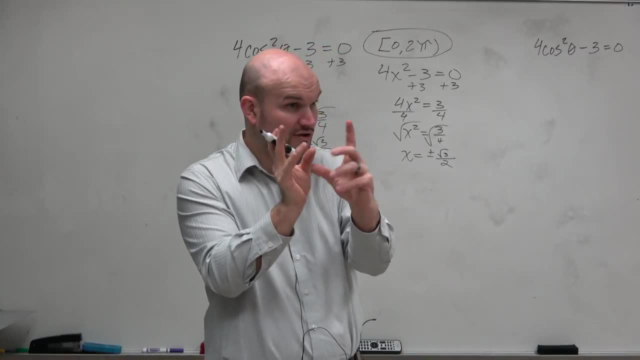 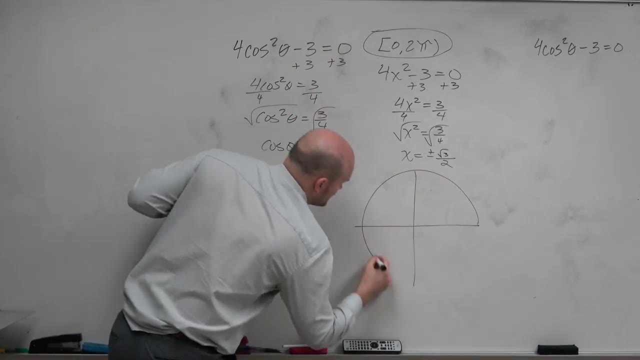 So we're not using inverse function, where we're just finding that one angle that fits within the domain. We're finding all of the solutions, So we go to our unit circle. I'm sorry, all the solutions between 0 and 2. 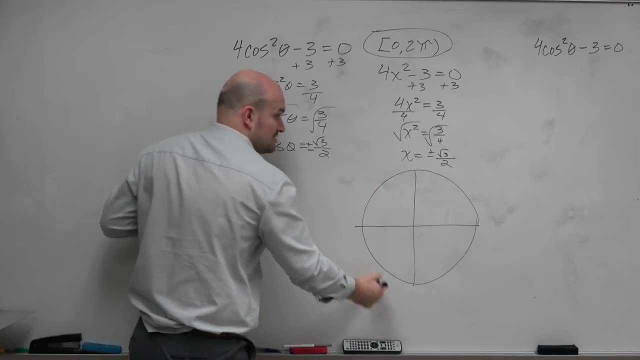 pi, which is basically one revolution of the unit circle right. Here's 0 to pi, Here's 0 to 2 pi. So it's basically finding all the values when cosine is equal to square root of 3,, 3 pi over 2.. 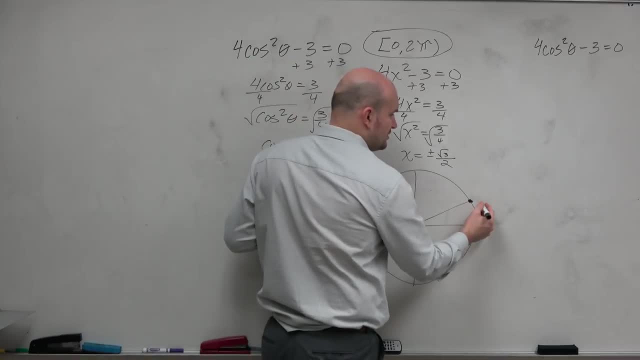 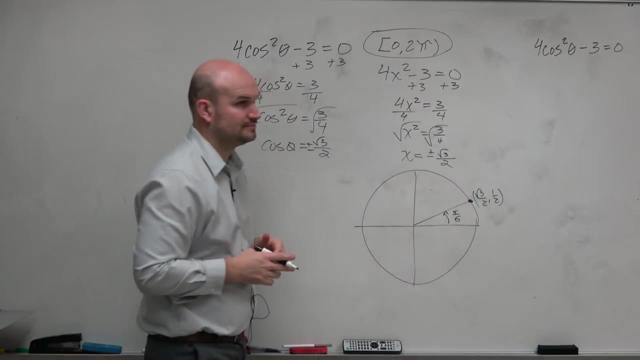 Now the way that I like to do this, or at least the way that I understand the unit circle, is- I know this coordinate point gives me that solution that I'm looking for. That answer is pi over 6, correct. And then if I want to find where are all the other angles, where? 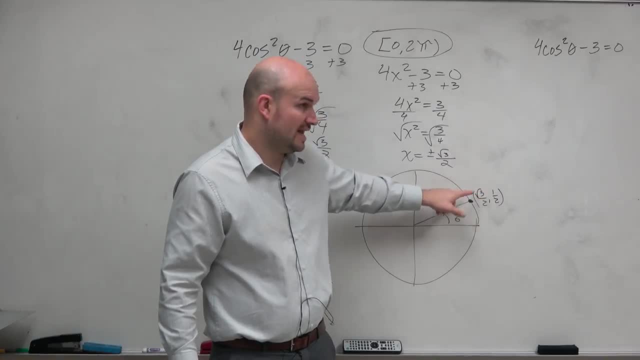 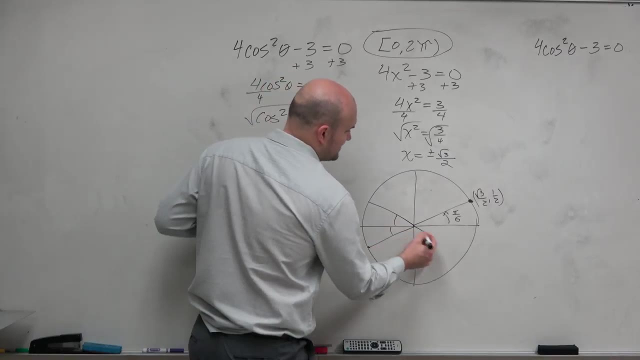 cosine is either equal to a positive square root of 3 over 2 or negative square root of 3 over 2, well, all these angles are going to all have the same reference angle. They all have a reference angle of pi over 6, yes, 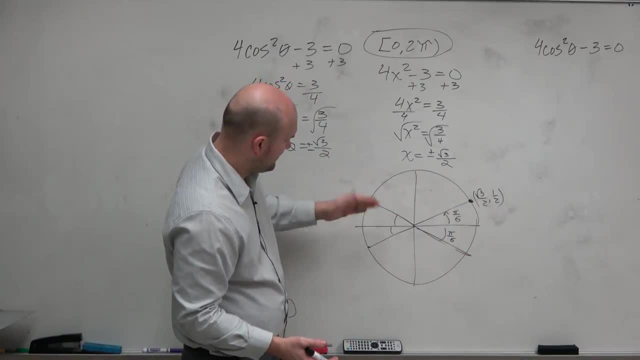 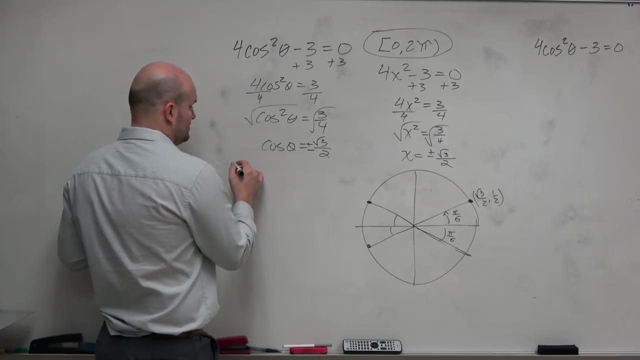 Because basically what these angles are is just a reflecting over here, reflecting down and reflecting down. So I'm not going to draw in all of these points, but you guys could say: theta equals, we know, pi over 6. Does anybody know what this angle is? 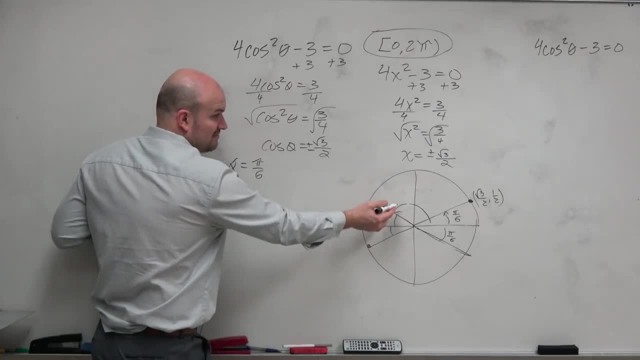 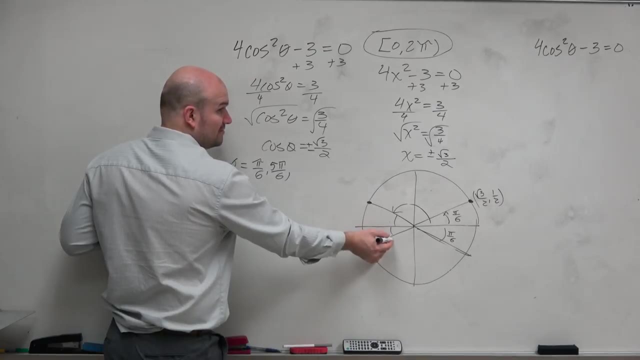 5 pi over 6, right, Because halfway around the circle is pi, or 6 pi over 6.. Subtract pi over 6, you're at 5 pi over 6.. This next angle is pi over 6 plus pi, which would be 7 pi. 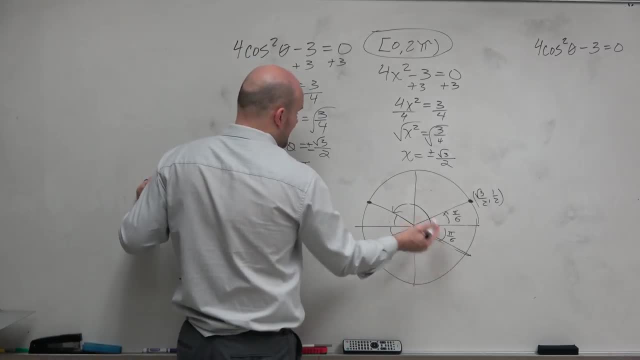 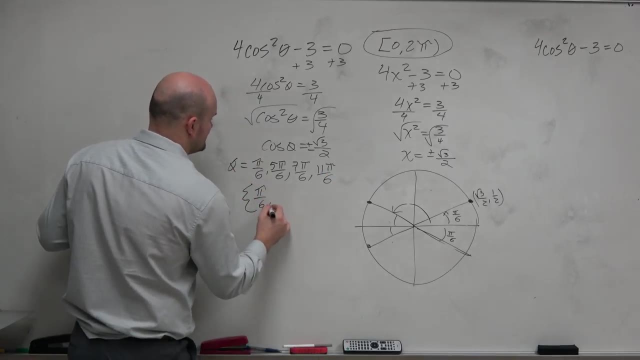 over 6.. And then this angle is pi over 6, short of 2 pi, which would be 11 pi over 6.. So you could see your answer written like this. You could also write your answer in set notation, just by using a set. 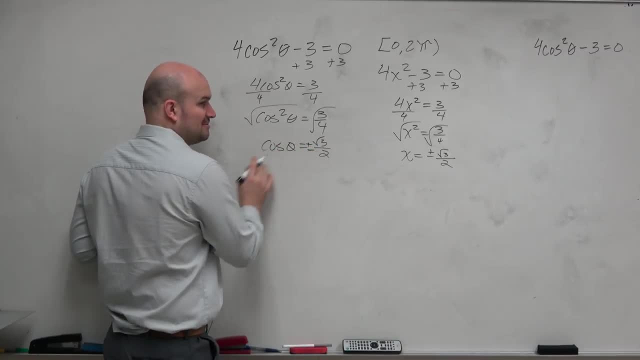 When I take the cosine of that angle, I get square root of 3 over- I'm sorry, plus or minus right. Plus or minus square root of 3 over 2. And then I have my constraint: 0 to 2 pi. 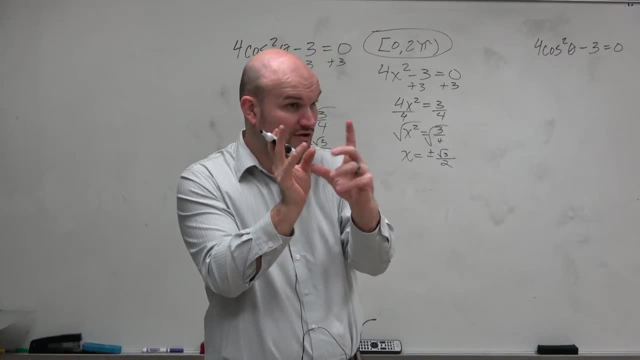 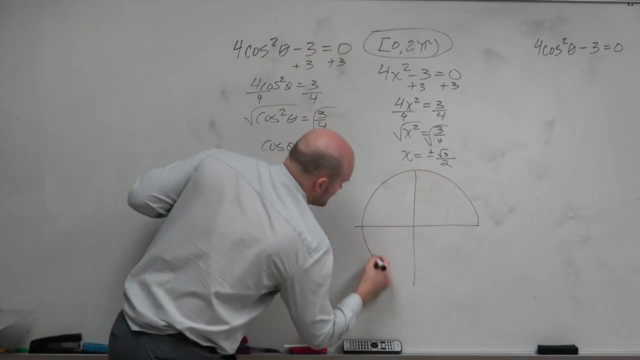 So we're not using inverse function, where we're just finding that one angle that fits within the domain. We're finding all of the solutions, So we go to our unit circle. I'm sorry, all the solutions between 0 and 2 pi. 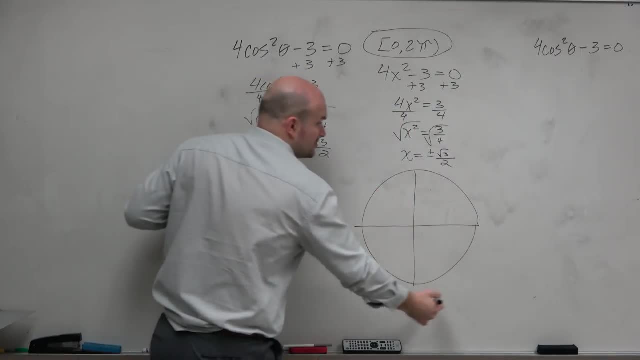 which is basically one revolution of the unit circle right. Here's 0 to pi, here's 0 to 2 pi. So it's basically finding all the values when cosine's equal to square root of 3 pi over 2.. 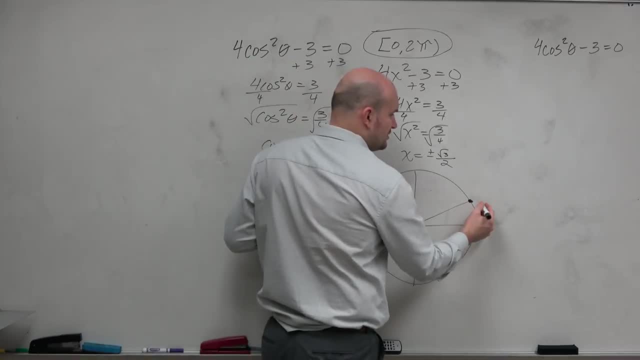 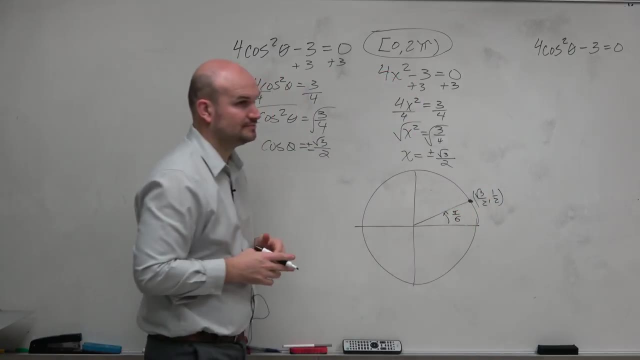 Now the way that I like to do this, or at least the way that I understand the unit circle, is- I know this coordinate point gives me that solution that I'm looking for. That answer is pi over 6, correct. And then if I want to find where are all the other angles? 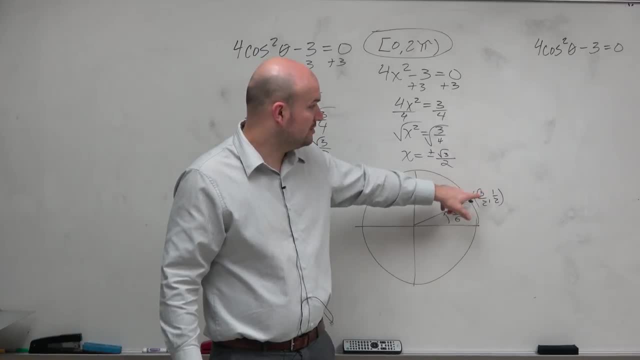 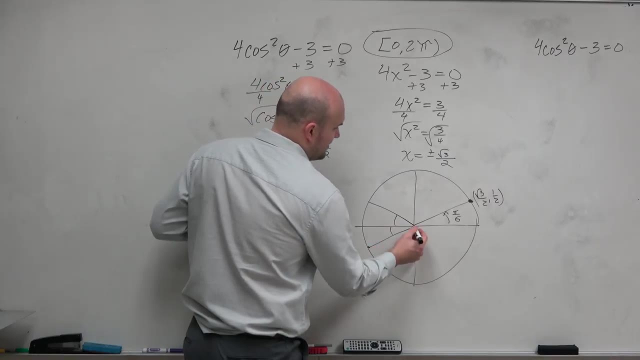 where cosine is either equal to a positive square root of 3 over 2 or negative square root of 3 over 2, well, all these angles are going to all have the same reference angle. They all have a reference angle of pi over 6, yes, 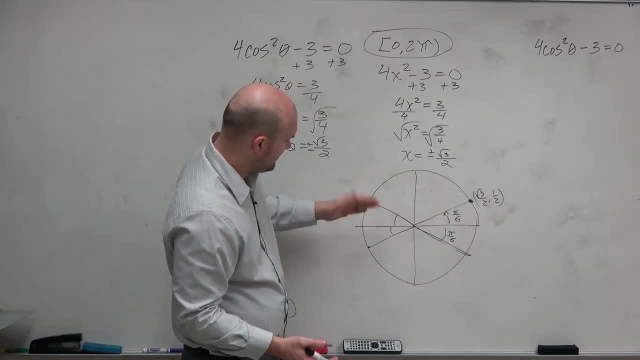 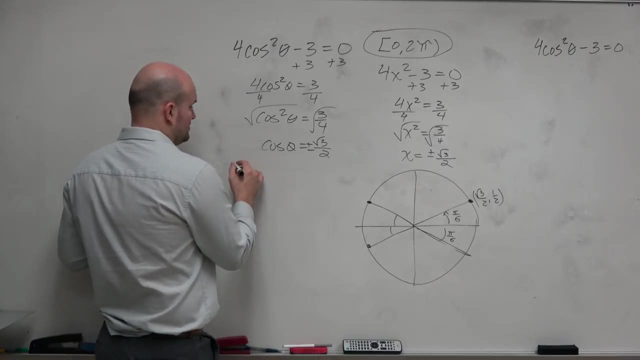 Because basically what these angles are is just a reflecting, Reflecting over here, reflecting down and reflecting down. So I'm not going to draw in all of these points, but you guys could say: theta equals, we know, pi over 6.. 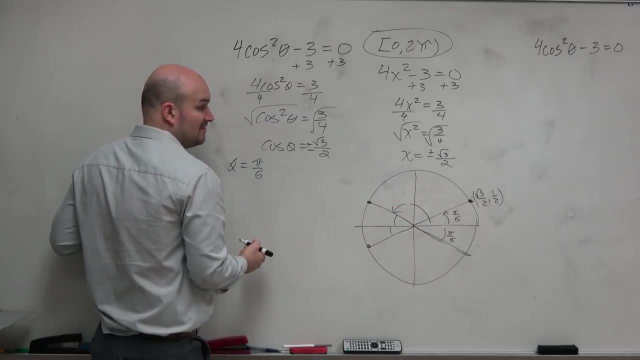 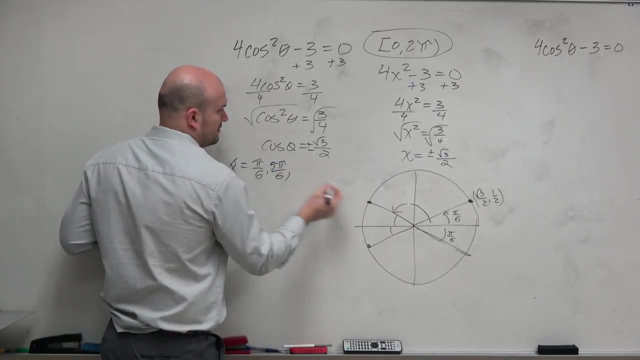 Does anybody know what this angle is? 5 pi over 6, right, Because halfway around the circle is pi over 6, pi over 6.. Subtract pi over 6, you're at 5 pi over 6.. This next angle is pi over 6 plus pi, which would be 7 pi. 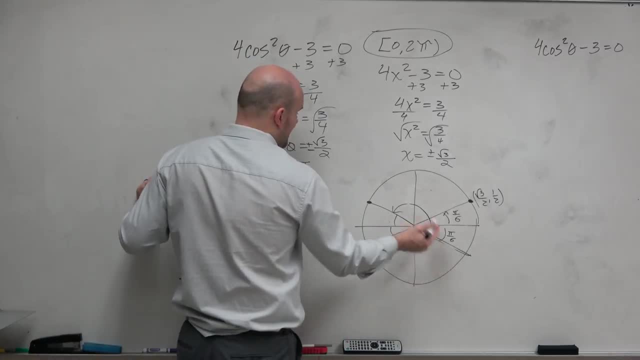 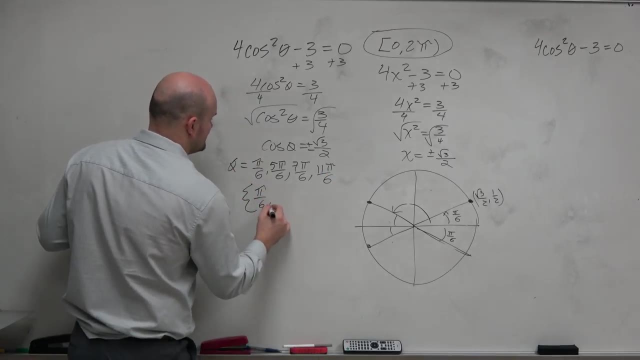 over 6.. And then this angle is pi over 6, short of 2 pi, which would be 11 pi over 6.. So you could see your answer written like this. You could also write your answer in set notation, just by using a set, and that's fine as well. 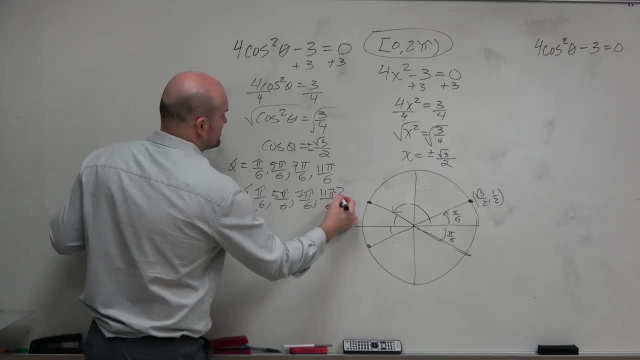 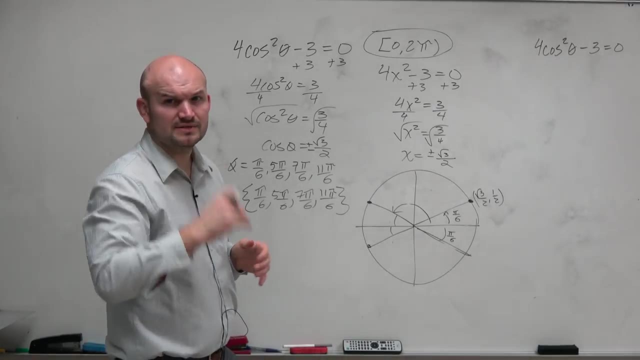 You'll see that often on your quiz something represented like that as well. Does that kind of make sense? Anybody have questions on how to find the other ones? Yes, If I said negative pi over 6 and negative 5 pi over 6,. 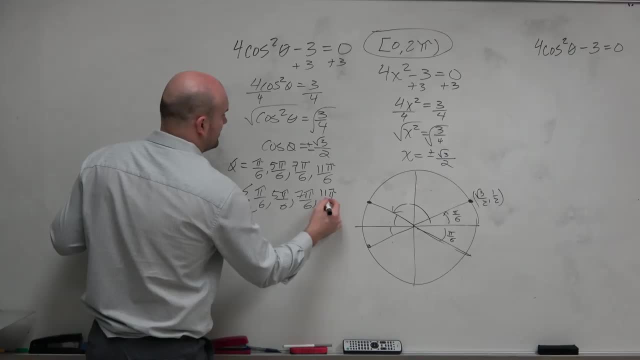 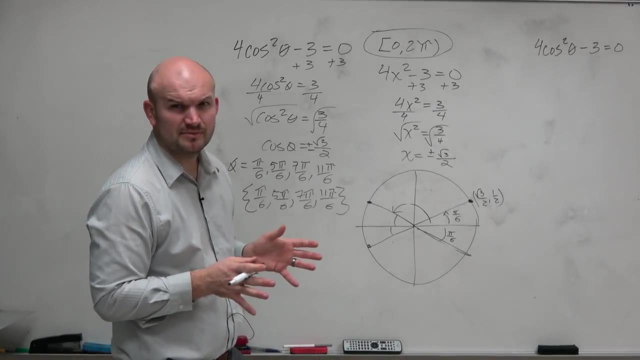 And that's fine as well. You'll see that often on your quiz. something represented like that as well. Does that kind of make sense? Anybody have questions on how to find the other ones? Yes, If I said negative pi over 6 and negative 5 pi over 6,.